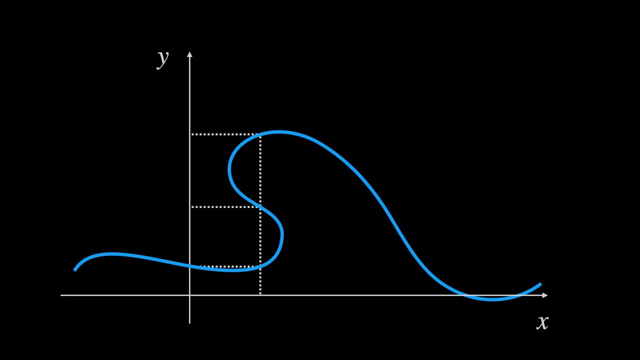 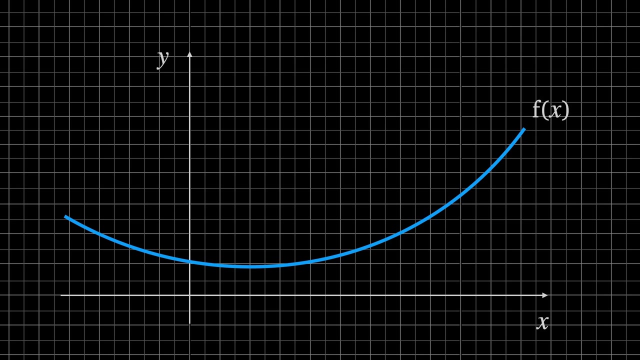 multiple outputs for a given input. So let rule 2 be that the output of a function should be unambiguous for all inputs. We'll first start with a graph of a function. Given that any point in this x- y plane represents a given x- y coordinate, One way to think about a function isn't to think of it as a rule, but 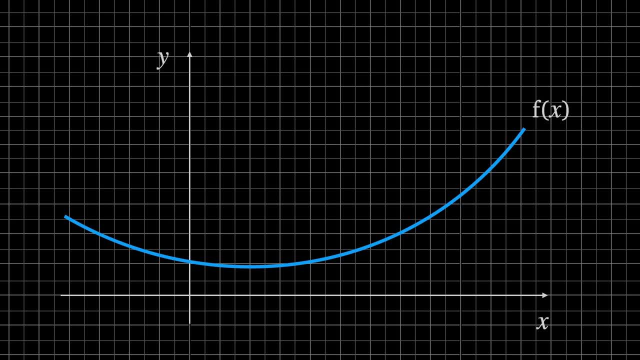 maybe a set of coordinates, Namely the set of coordinates represented by this blue line. But then what is the set of coordinates that make up the x? y plane? Well, we now have to introduce the product of two sets. The product of two sets is the set of coordinates that make up the x? y plane. 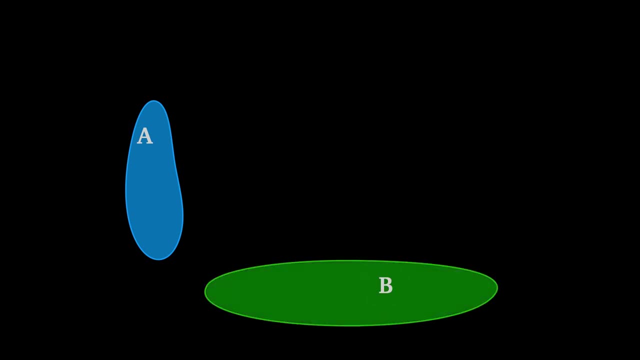 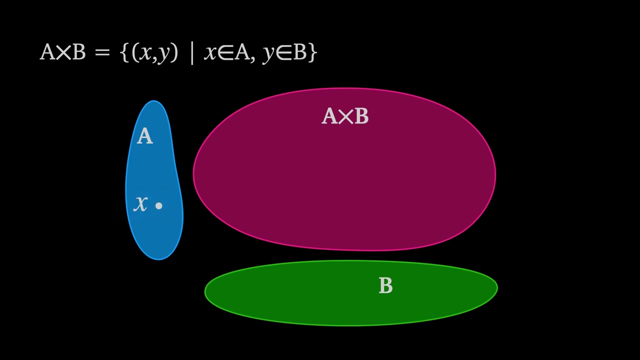 Given a set a and a set b, the product of a and b, a cross b, is the set of all ordered pairs x and y, such that x is in a and y is in b. That is for all elements, x in a and y in b. 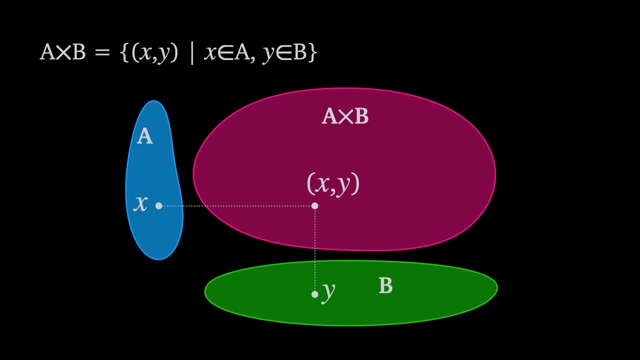 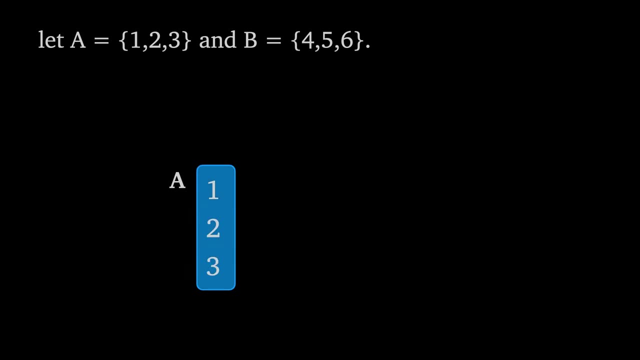 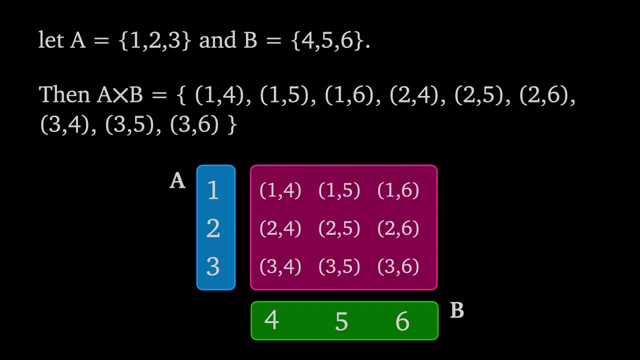 there'll be a corresponding element x, y in a cross b. For example, let a be the set containing one, two and three and let b be the set containing four, five and six. Then a cross b is the set of the ordered pairs: one, four, one, five, one, six, two, four, two, five, two, six and three, four, three, five. 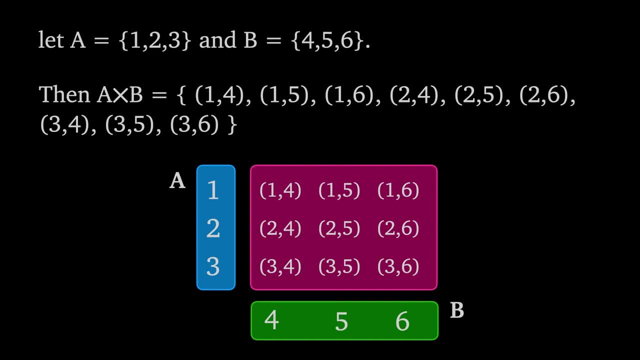 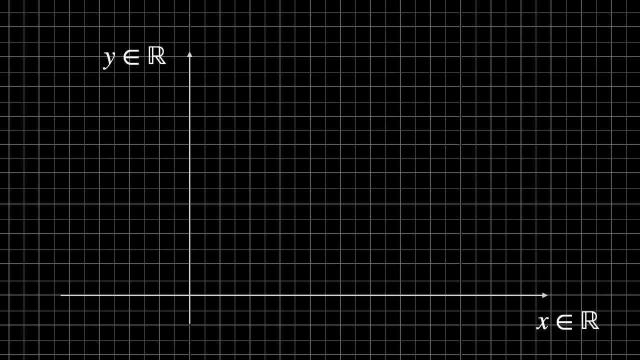 three, six, Visualizing the sets and their product. this way gives a nice insight into how the x? y plane is formed of the product of two sets. In this case, we often have the x? y axes representing the set of x and y belonging to the real numbers, and so, in that respect, the x? y plane is a set r cross. 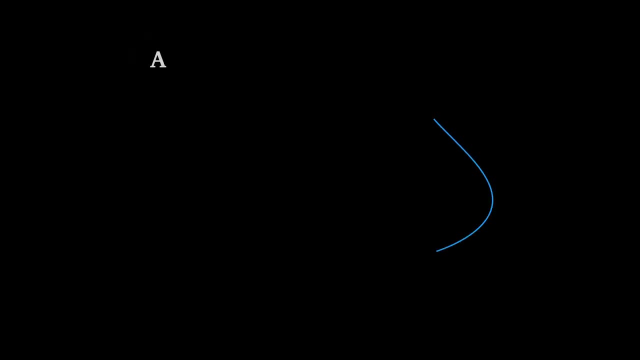 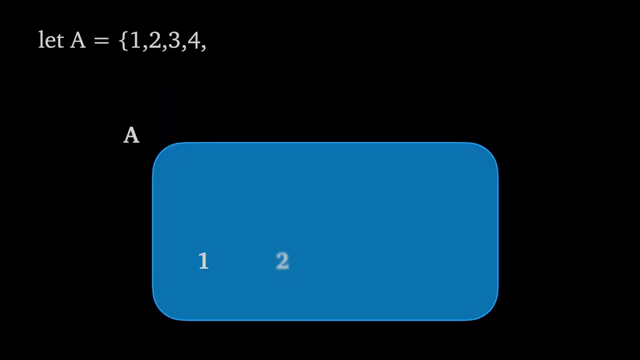 b. The next concept we need to introduce is the relation. It's possible to divide a set into two parts if something about the elements can be evaluated as true or false. Take, for example, the set a of numbers one to eight. The expression x in a, such that x is less than four, divides a. 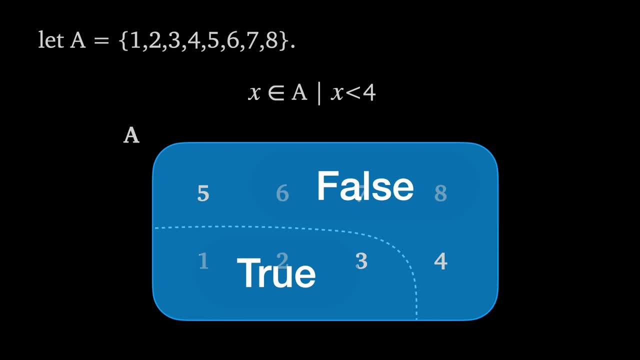 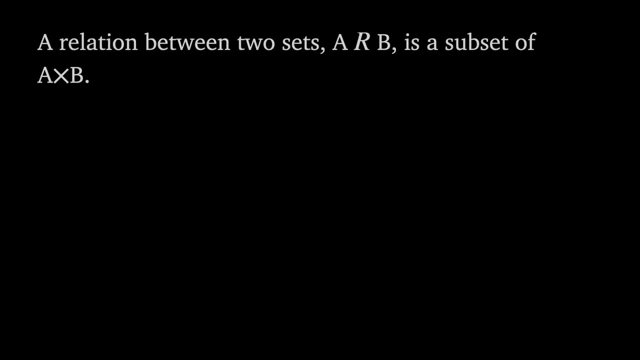 set into two subsets: The subset for which this is true, containing one, two and three, and the subset for which this is false. We define a relation on sets a and b. subset of a cross b. Specifically, it's the set of those ordered pairs x and y, such that some 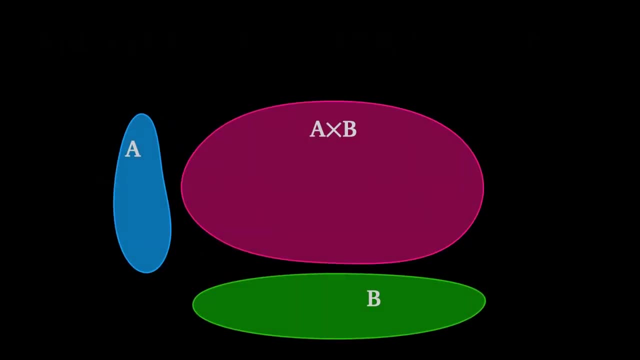 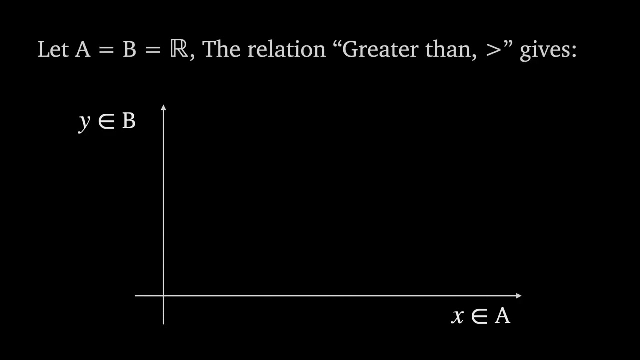 statement comparing x and y holds true. For example, the relation greater than applied to sets a and b gives a set of all ordered pairs x and y in a cross b, such that x is greater than y. If we let a and b be the set of real numbers, then the relation greater than 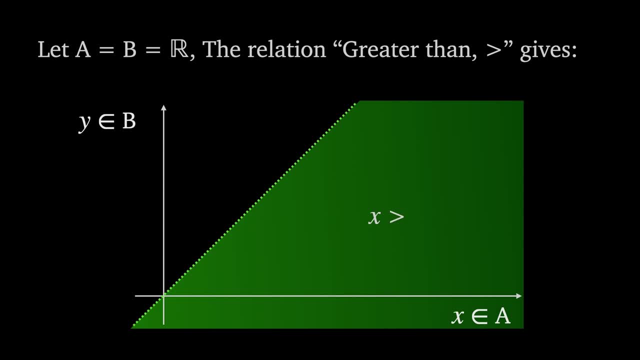 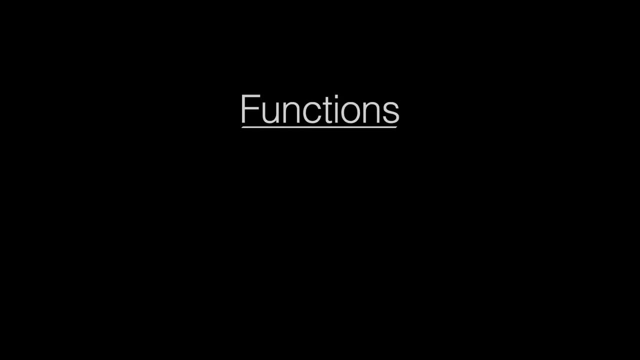 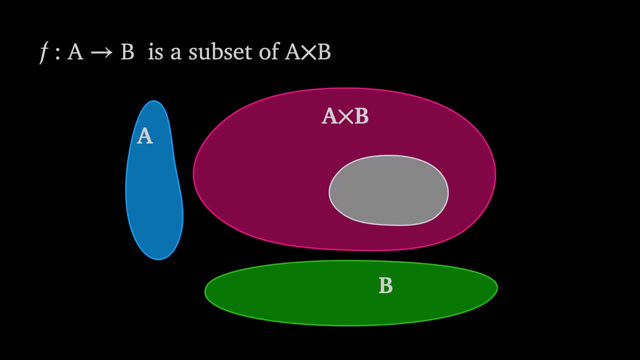 gives the region of the x- y plane where x is greater than y. This is the region below the line. y equals x. We're now ready to write down the definition of a function. We use the concept of a relation to define a function, The relation itself being that. 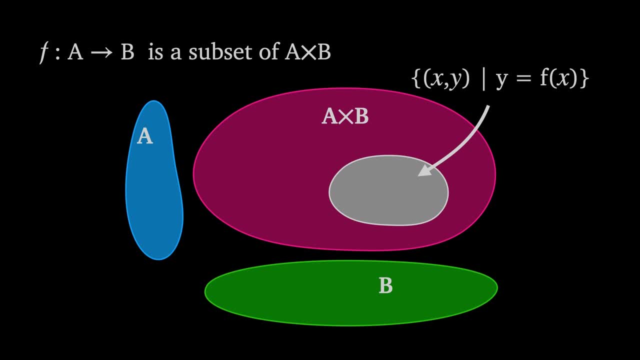 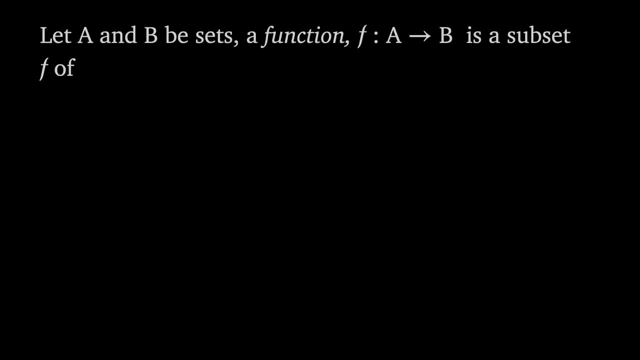 y is equal to f of x. However, f of x must follow some rules in order to avoid some of the issues we saw earlier. Let a and b be sets A function. f from a to b is a subset. f of a cross b such that 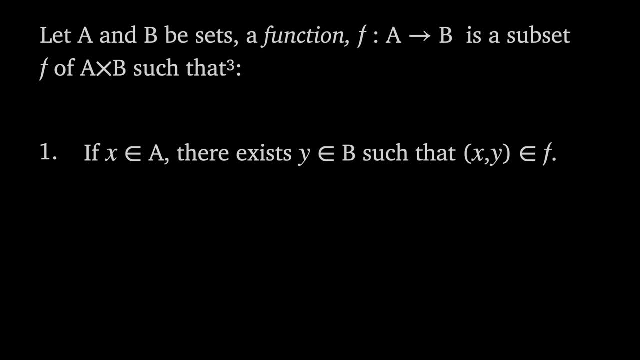 if x is in a there exists y in b, such that the ordered pair x and y is in f, And if for x in a there exists y and z in b, such that x and y is in f and x and z is in f. 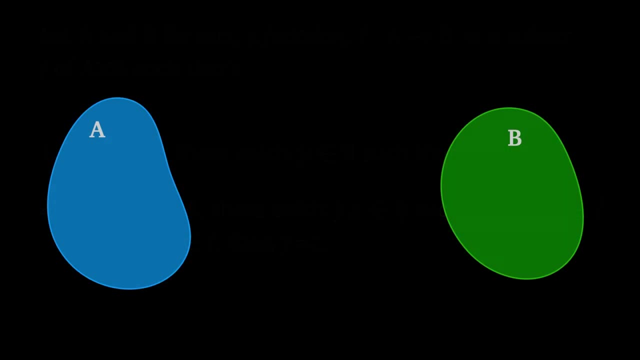 then y is equal to z. These two rules are a little bit cryptic, so let me explain exactly what they mean. A function from set a to set b maps a onto a subset of set. b- main of the function, and b the co-domain Rule. one ensures that given any element x in a there is 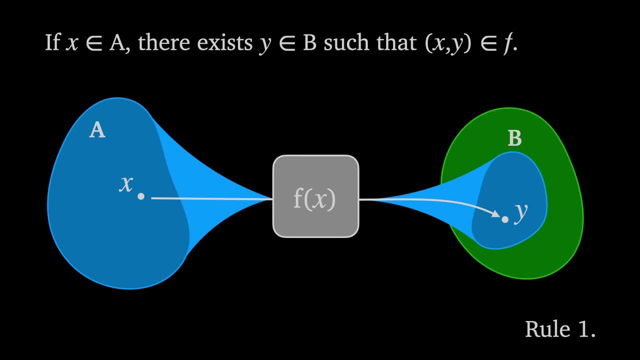 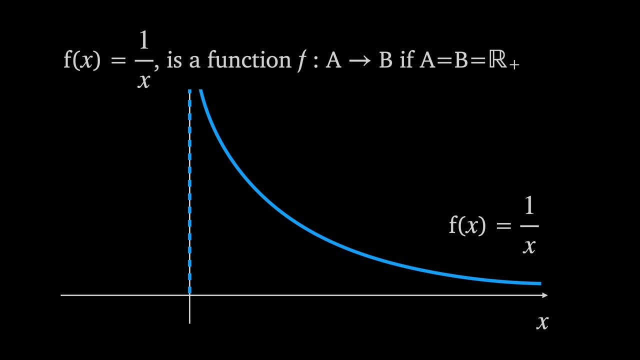 always a corresponding y in b, such that x and y is in f. In everyday language, that means the function must give a valid output for every value put into it. and so, coming back to the function, 1 over x, which isn't defined at x, equals 0. we see now that restricting the domain of f so that it doesn't 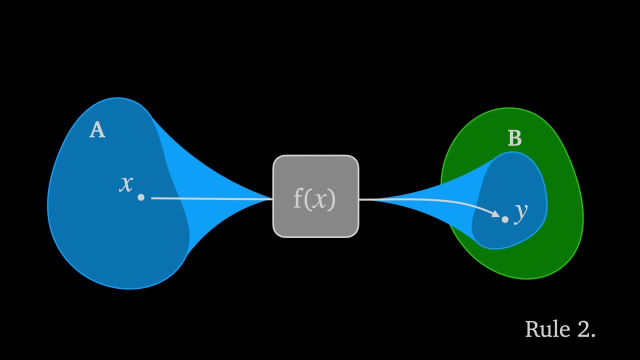 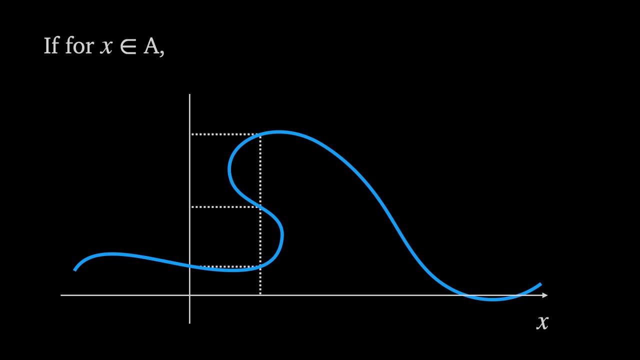 include 0 solves this problem. By rule 2, we also prevent a single value from the domain a be mapped onto two distinct values- y and z- in the codomain b. this prevents us from allowing cases such as this with multiple values again, if for a given x there exists y and z, such that